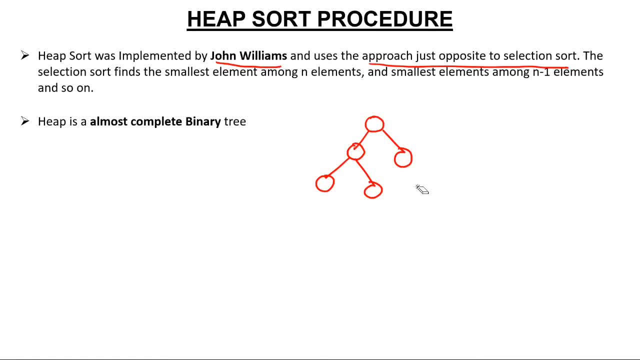 here, Fifth will come here, Sixth cannot come here. First of all left node will come This, and then this, Then this. It is not possible. No. First left child, then right child For every node. first left child, then right child For every node. first left child will be completed, Then right child. 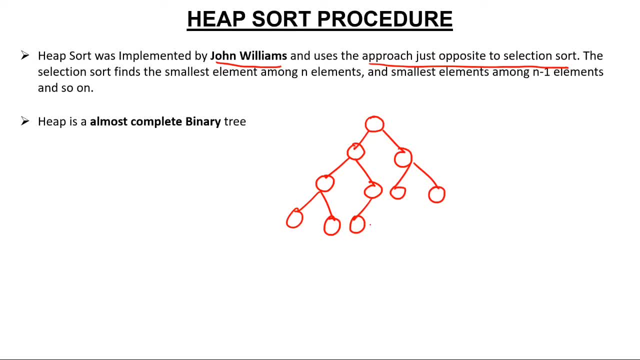 child will be completed, Fine, Okay, So is this a complete binary tree or almost complete binary tree? Yes, Is this a complete binary tree or almost complete binary tree. So this Heap is almost complete binary tree, or you can say complete binary tree In some books. 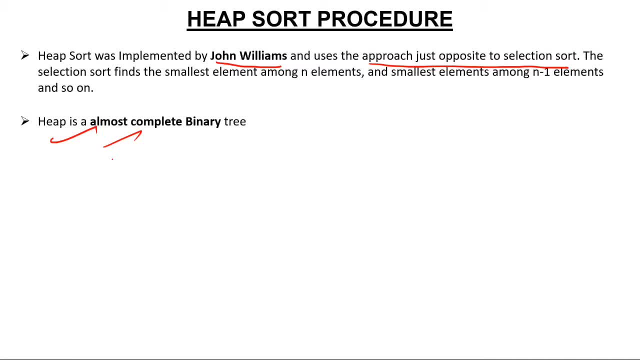 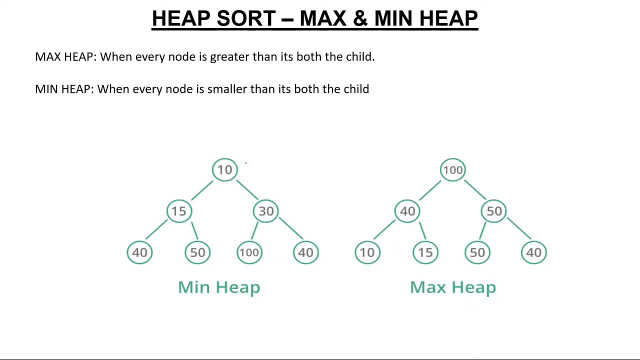 it is said as complete binary tree. In some books it is said as almost complete binary tree. Fine, Okay, Now what is MaxHeap and MinHeap? We have already discussed What is MinHeap When? if you consider any node, then any that node should be less than its both the child Is. this is less than. 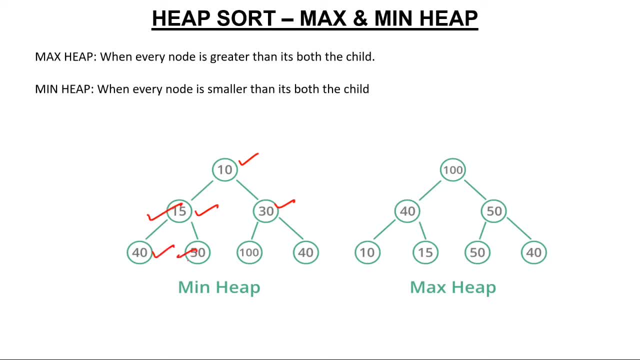 both the child? Yes, If you consider this node, is this node less than both the child? Yes, If you consider this node, is this node less than both the child? Yes, So this is MinHeap. Now MaxHeap is just opposite to MinHeap. You consider any node, it should be greater. 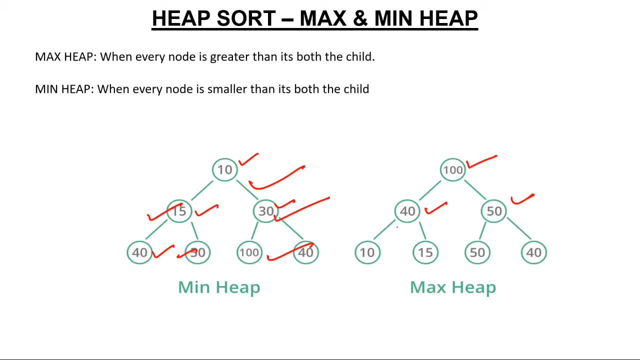 than its both the child? Fine. Is this node is greater than both the child? Yes. Is this node greater than both the child? Yes. Is this node greater than both the child? Yes. Is this node greater than both the child? Yes. So this is MaxHeap and this is MinHeap. Fine, 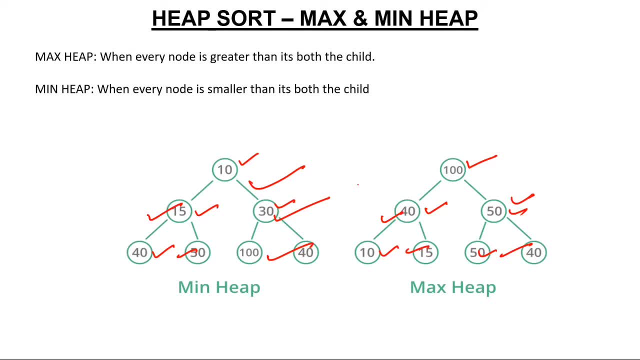 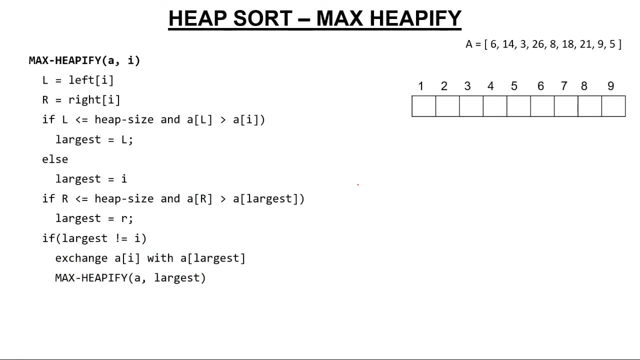 So this is MaxHeap and MinHeap, and you have to keep this particular thing in mind and in my previous video I have already explained you how to create MaxHeap and MinHeap. So let's move further and see the algorithm of Heapify. That is, what is Max? How to Heapify. 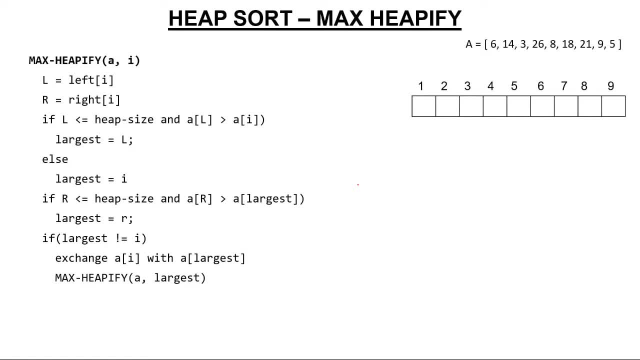 that is how to create MaxHeap and MinHeap. So this is the algorithm, So which we have already discussed, but my job is to explain you. So you have given an array. Let me put the values in an array, which is 6,, 14,, 15,, 16,, 17,, 18,, 19,, 20,, 21,, 22,, 23,, 24,, 25,, 26,, 27,. 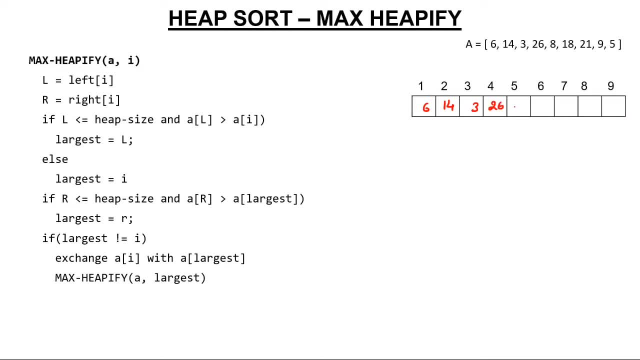 28,, 29,, 30,, 31,, 32,, 33,, 34,, 35,, 36.. This is a simple array: 8,, 18,, 21,, 9 and 5.. Let me make a tree of this array: 6,, 14,, 3,, 26,, 8,, 18,, 26,, 8,, 18,, 21.. Then we have 9,, then 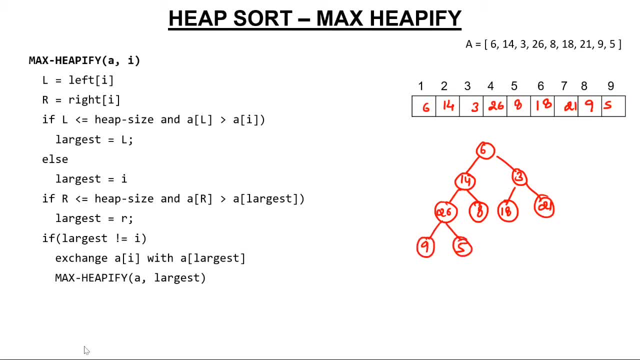 we have 5.. Fine, So we have created a tree. Now let me change the color of my pen. Now, let's make a tree. So we have created a tree, Now let me change the color of my pen. Now me explain: is this a max heap? no, this is not a max heap. so how to do max heapify, which i have? 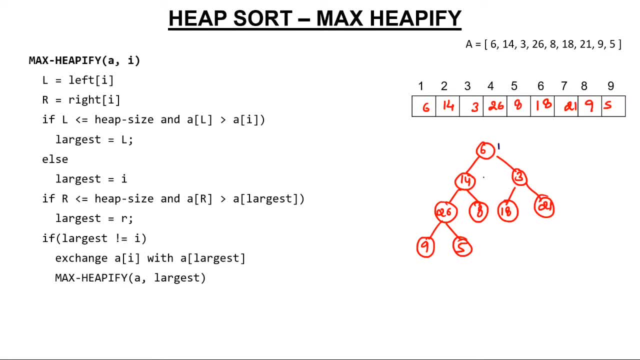 already explained you that, if you, if i consider the index, this is first index, this is second index, this is third index, this is fourth. you can match from array: fifth index, sixth index, seventh index, eighth index, ninth index. what i have to do, i have to start from what i have to do, i have to start. 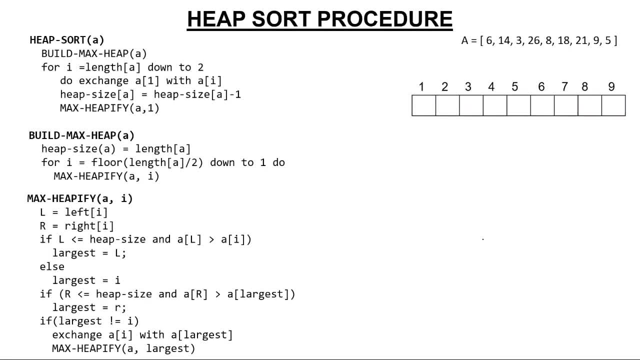 from, so let's see the algorithm first. okay, this is the array, so let's see the algorithm. uh, suppose 6, 14, 3, 26, 8, 18, 21, 9 and 5? what you did first of all. your job is to do. your job is to sort this. 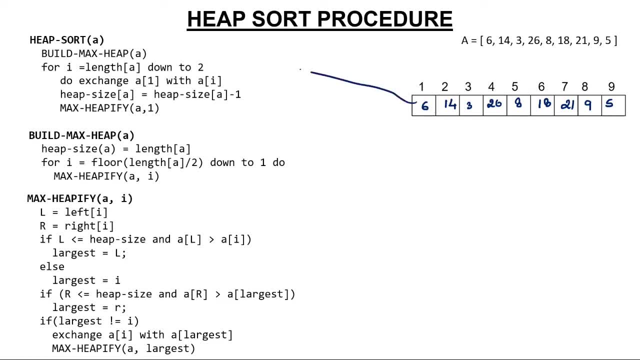 element. so, in order to sort this element, what you did? you simply called heap sort. you said: heap sort, take this array and sort it. so heapshot said: so see what heap sort said. heap sort said, instead of coming to me, fine, you came to me, but what i'll do? i'll first call. 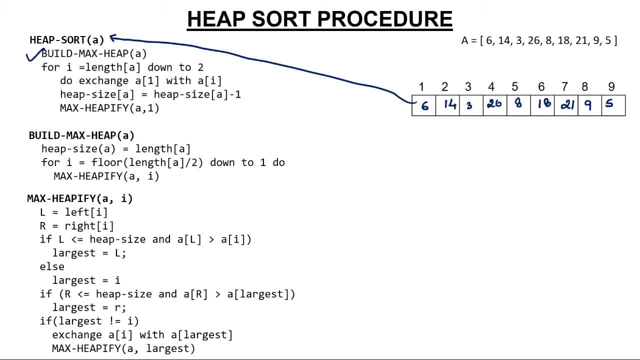 maxi. so this is what? so what this is saying? this function is saying, instead of coming to me, yes, you just go and call build maxi. so what heaps are good? so heapshot, you know, took the entire array which is passed to him and the pass the same array to build maxi. so i'll again jump. 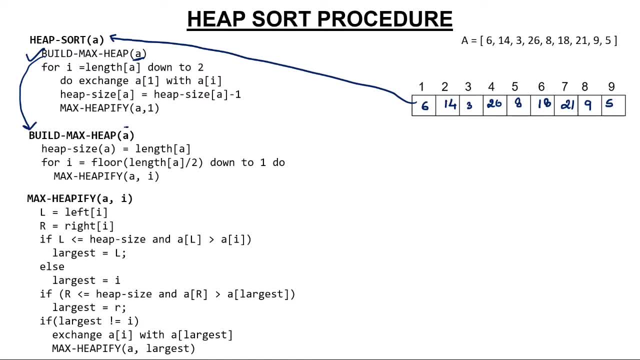 to the new definition of build, maxi and i have given this array. so what i'm doing, what heapshot is saying, so i'll heap sort only when, when it will be either maxi or mini. so since i am considering it, so it has called a new function which is called maxi. so what maxi will do, it will calculate the. 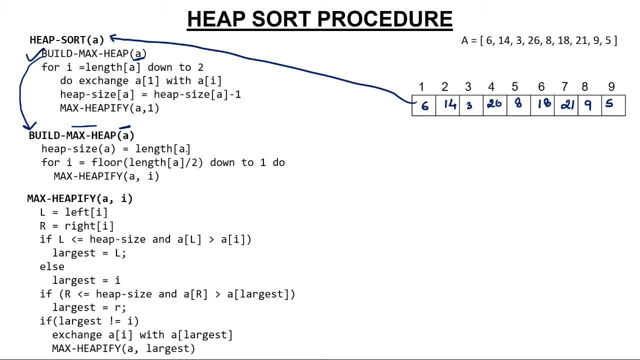 size of heat. so heap size of a is equal to length of a. so what is length of a? 9, so it will become 9. fine, okay. so from where i have to stack, which i have already explained from half, what is length? 9 by 2, and the 9 by 2 floor value is 4. so i will start from 4 till 1. so i will start from 4. this 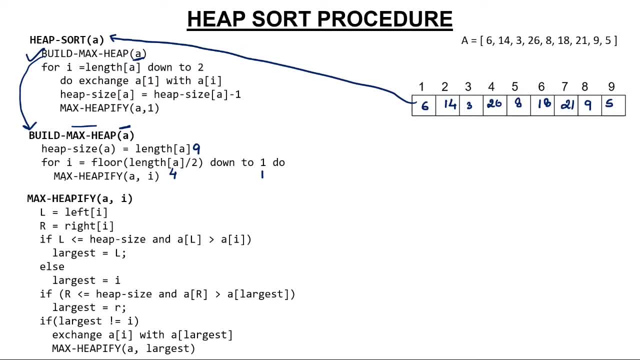 loop will start from 4 to 1.. fine, okay, now let's see what i'm doing. is thought i'm calling what i'm calling max heapify. see, i'm calling max heapify a i, what is a, the entire array and what is i? 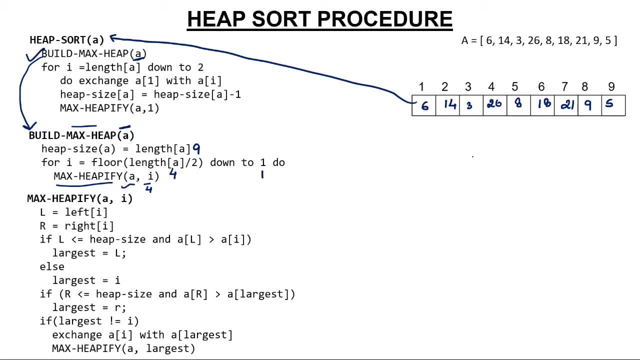 4, so i'm giving an entire and 4, so let me make a tree over here. fine, okay. so 6- 14, we have 3. 6, 14, we have 3, we have 3, then we have 26, we have 8. 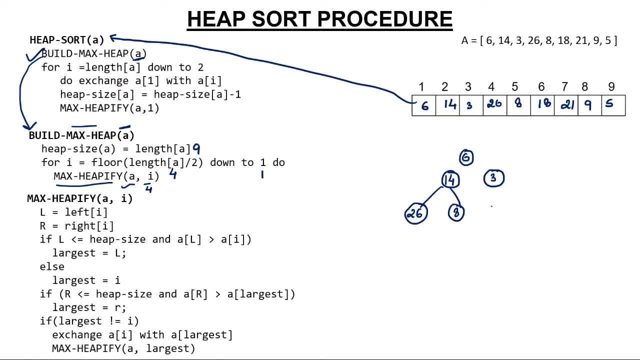 26, we have 8, then we have, uh, 18, then we have 21, then we have 9 and then we have 5. fine, okay, now what to do is that i'm calling this maxcp5. see, this maxcpy will create maxi. fine, so what it will? 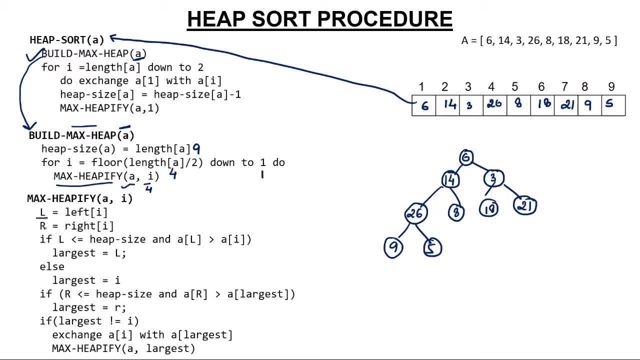 do. it will what it will. it will, uh, find the left and it will find the right. so in for i make left what is left of i this. so this will become l and this will become r. so if i tell you the formula, the formula is very simple. suppose i am asking what will be the left child of 26 and what will 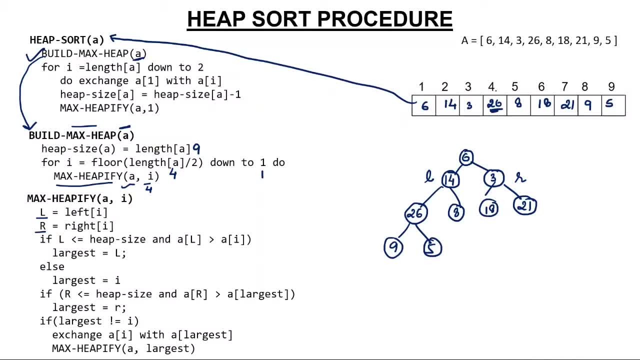 be the right child of 26.. so you just find out the index of 26, which is 4.. so left child of any node is 2i. left child of any node is 2 child, 2i. right child of any node is 2i plus 1.. so what is i? 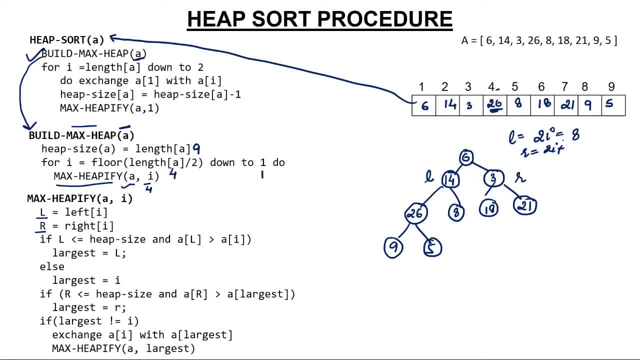 4. so 2 into 4 is what? 8 if you see the eighth index. so if you see the eighth index, which is 9, so the eighth index has 9, so left child of left child of 26 is 9.. you can clearly see yes. 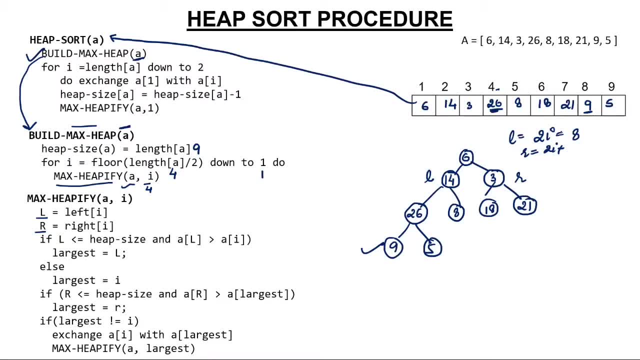 left child of 26 is 9.. if i have to find in in an array only without having 3, which is the right child of 26, 26, that is what is the index of 26: 4, 2, 2 into 4 plus 1, which is what: 9, so at 9th index. 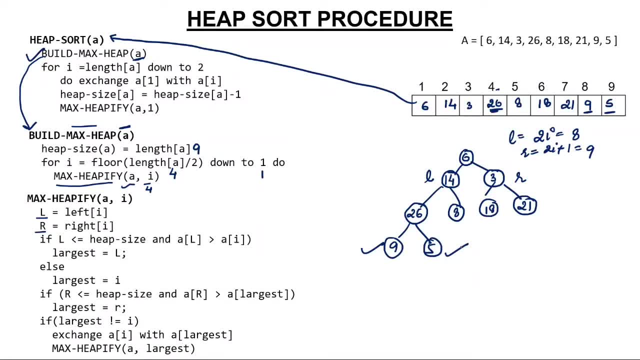 you will find 5, so 5 will be the right child. yes, exactly right, which is very correct. fine, so if, why i'm using 2i and 2i plus 1? because my array is starting from 1.. what if my, if my arrays is starting from 0, then left child formula will be 2i plus 1.. i'll simply increment. 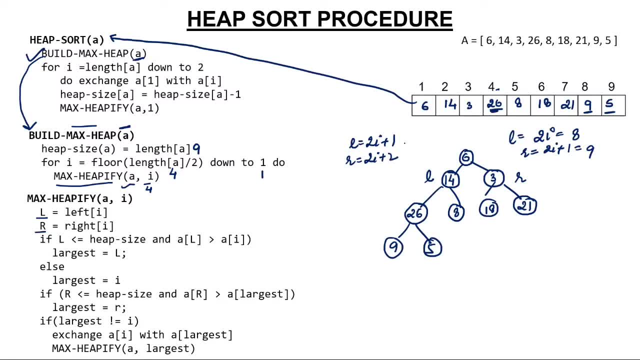 and right child formula will be 2i plus 2.. since we are starting our array from 1, so we'll consider this formula fine. okay now. so what is l how we have calculated? l hope you understood, so l will be left. i r will be right, which i have put now. what we'll see is: now: let me make the index also. 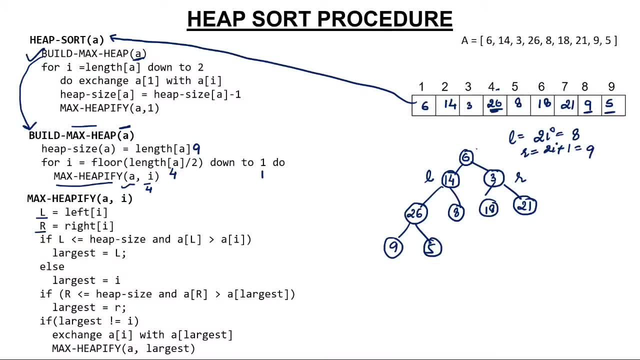 let me make the index also. it will become easy for you to understand. this is first index, this is this, one is third index, this one is fourth. you can match from array fifth index, sixth index, 7th, 8th and 9th index. fine, okay, so what i'll do is what? what i'll do, i'll check, is left. left is what. 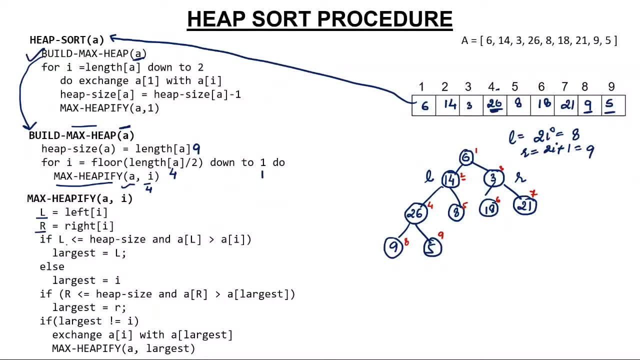 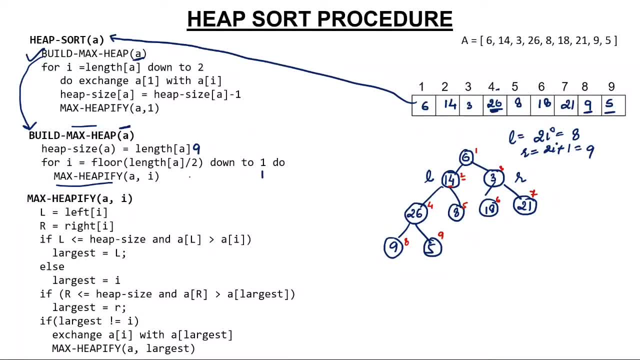 Okay, Fine, Okay, Okay, Okay. So let's, since we have to start from four, since we have to start from four to one. So what I'll pass, I'll pass a and I. what I'll pass is a and I. So what I'll pass is a and I. So what I'll pass is a and I. 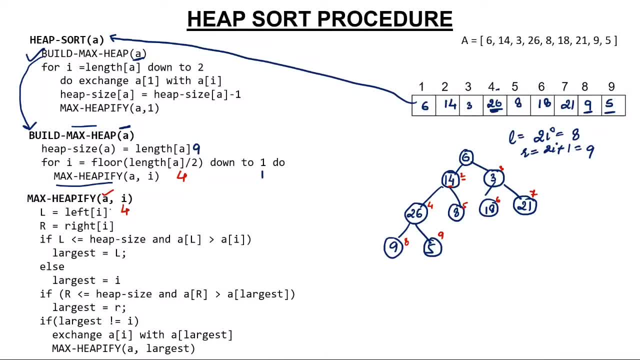 What is I? Four, So L will from. I'll start from four. So what is four? I will come here. What will become L? This will become L, And what will become R? This will become R. Now I'll check. 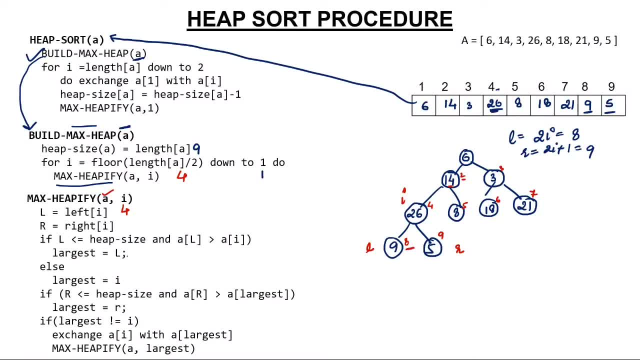 is L less than heap size? What is L? Eight? L is always an index. Is eight, Yes? Is AL? What is AL Which is nine? What is value over there? Nine Is nine is greater than AI A. what is AI What? 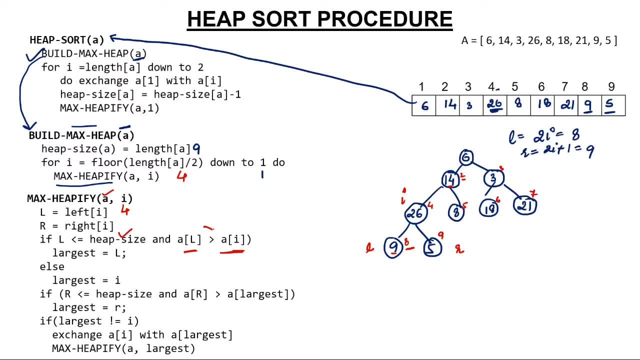 is AI 26.. No, nine is not. So this is true, but this is false. So entire everything is false. Fine, Okay, Now I'll go to the else part And what will make? I'll make largest to I What is. 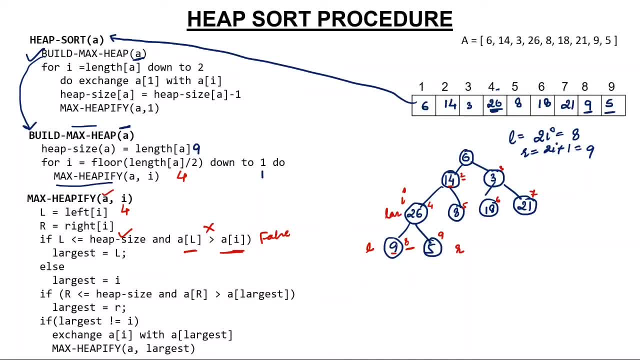 I Fourth. So which is largest? 26 is largest. Which is, which is very true, No, among 26 and nine, which one is largest? 26 is largest. Now I'll come to this part. Is R? What is R? R is? 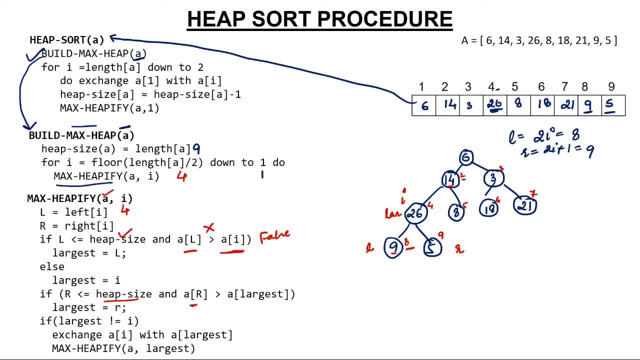 representing nine. Is nine less than heap size? Yes, Is AR. value of AR is what? Five? Is five greater than A largest? What is A largest? 26.. No, five is not. This is again false. So if this: 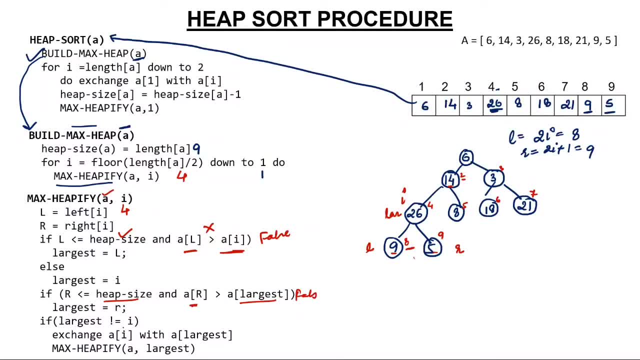 is false. I'll not change. largest Now, if I'll see, is largest not equal to I? No, this is again false. Largest is equal to I because I and largest both are at same index, That is, at index four. So if they are both at, 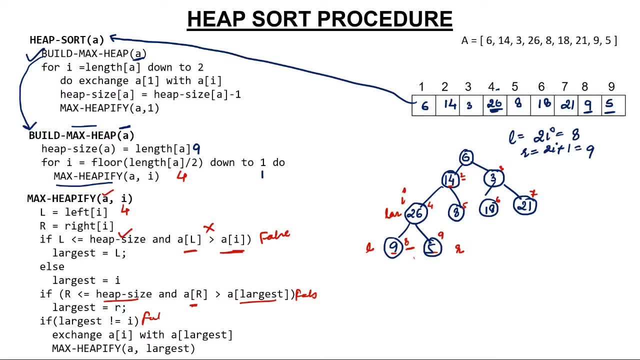 same index. why will I exchange it? I will not exchange it. Fine, So 26, it's is at correct position. So now, what will happen? I'll again what will happen: Loop will get terminated. This function will get terminated. Where I'll go? I'll simply go and decrement, I'll decrement, I. 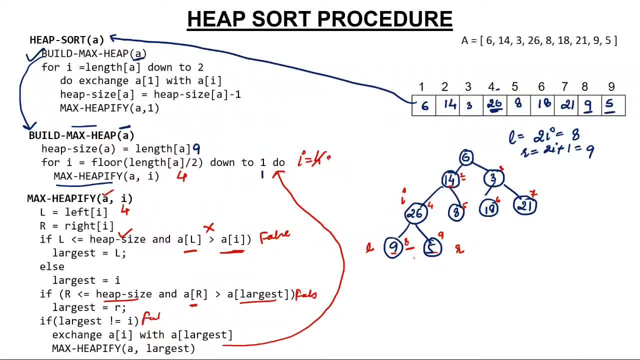 So now I will become first value of: I was four, I will become three, So again I'll call this function. Again I'll call this function A and give I: I is three, So I will become three. So what I'll do now, what I'll do now, I'll start. 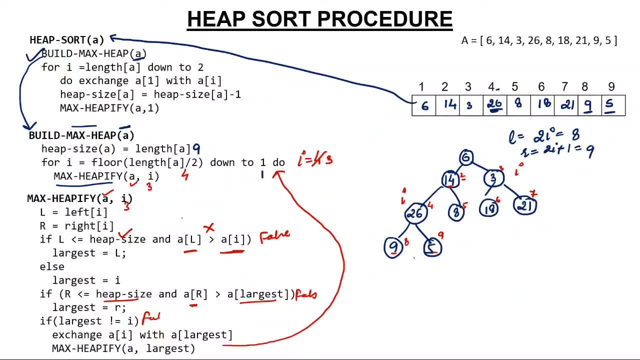 from what I'll start from three, That is this. So what will be L? This will be L left of I, This will be R right of I. So L is at sixth index, Right is at seventh index Is L, that is six. 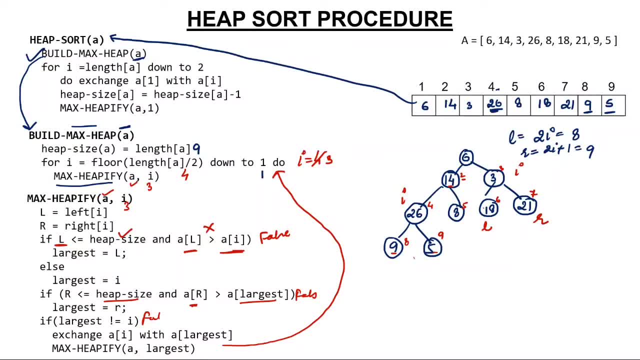 less than heap size? Yes, Is AL AL. what is AL? 18.. Is 18 is greater than AI Three? Yes, So this is greater. Now both the condition are true. So this will condition will become true. So which will be the largest? will become L. So among these two elements, 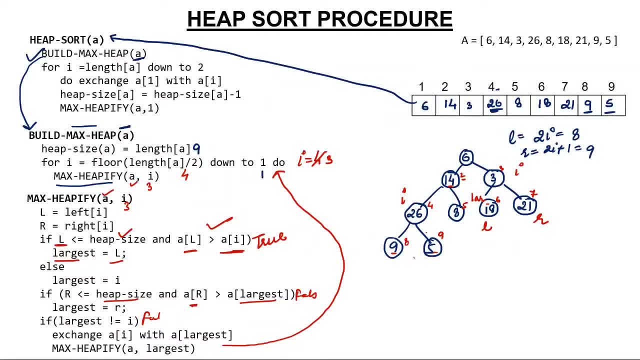 which is largest, So I'm making this as largest, So this 18 is largest, Fine, But still we have one element to be considered Fine, So I'll I'll not move to the else one. I'll again check- Is R. 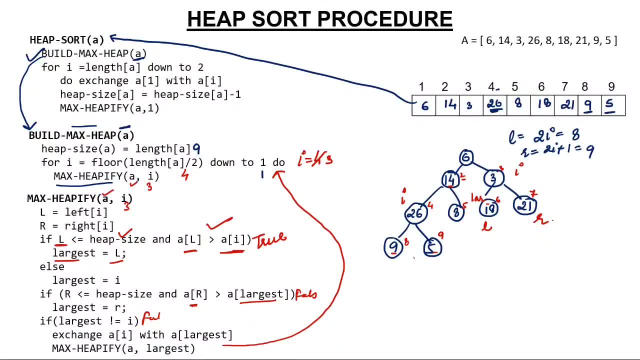 less than heap size. Yes, R is seven and seven is less than heap size. Heap size is nine. Is AR? what is AR? 21 is greater than A largest, which is largest, 18.. Yes, So this is also true. This is also true. So the entire condition become true. So largest will. 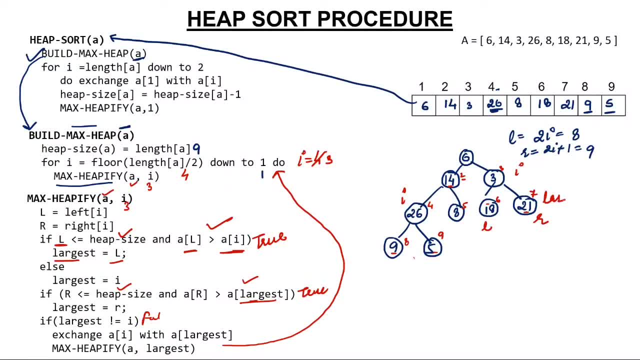 become R, So this is not largest now, This is largest. Fine, So, and you can clearly see that among these three elements, which is largest? 21 is largest. Now I will check: Is largest and I not equal? Yes, Largest and I are not equal, because I is at index three. Largest is at index seven. 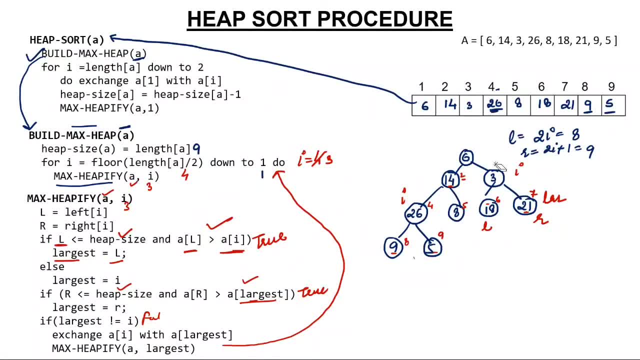 So this: they are not equal. So what I'll do? I'll exchange AI and A largest. So what will happen? What will happen? 21 will come here, Three will come here, Fine, Okay, And which I already told. 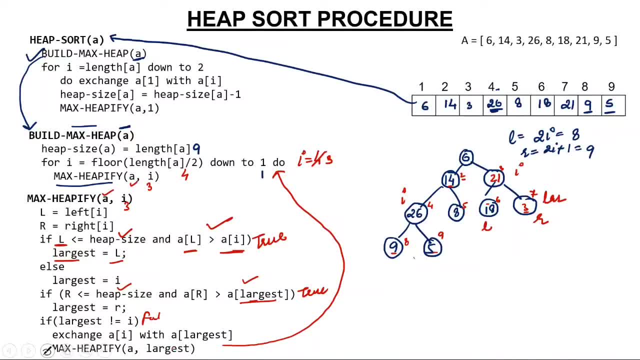 this. Now, again, I will call max heapify function with value A and largest, because the one which is largest will become I. So what will happen? See A largest, what is largest? Largest is at seven. No, this one was largest, So this largest, I'll pass this largest. So I'm again calling A. 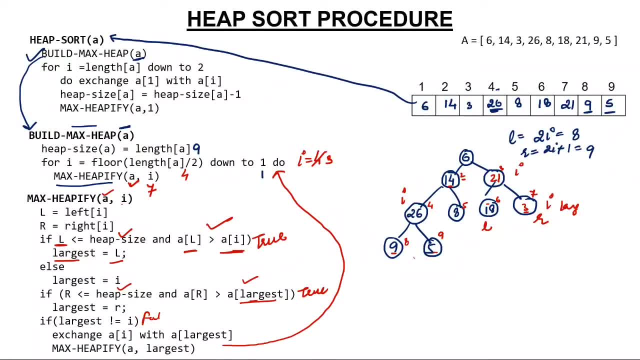 with what is the value of a largest Seven. So again it will come: call A seven. L will become left I. Is there any left? Is there any left? No, there is no left. And if I have to calculate using this formula, then what will be the value of A largest? I will call A largest. I will call. 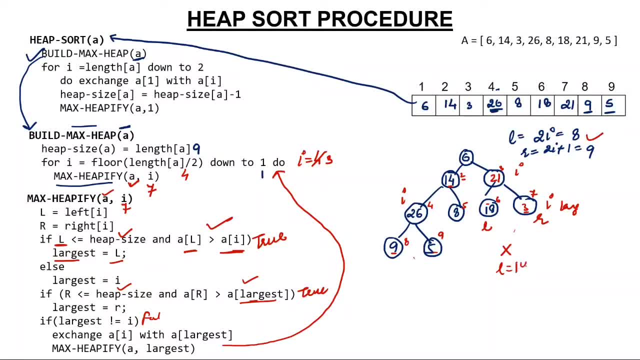 left two into I, That is, two into seven, So L will have 14 and right will have 15.. Since there is no index of 14 and 15, so condition will become false. See, this Is L equal to less than heap. 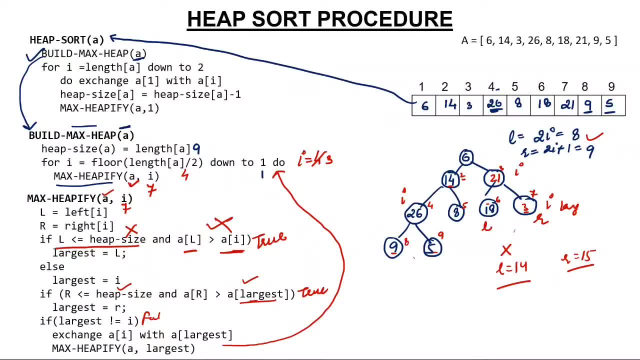 size: No, false. If this is false, I'll not execute this, So this entire will become false. Again, I'll come. Is R less than heap size? No, So again, I'll not check this, So this will become. 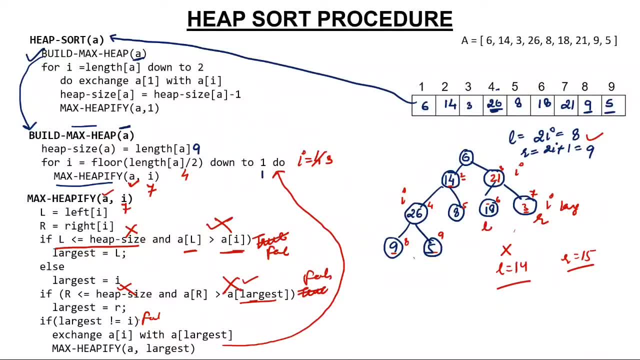 false. So is largest and I not equal? No, Largest and I are equal because I is also here. Largest is also here, Since both are there. so I'll not exchange also and not move inside this if block, Fine. So if I'll not move inside this, if block, what will happen? What will actually happen? I'll. 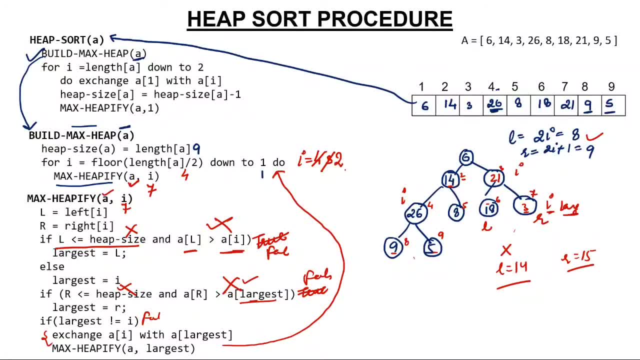 again move back and increment decrement value of I from three to two, you know, because I will now become two. So what will happen now? This? I will become this, I will become two, So I will come here. Fine, Okay, See how we are maximizing the entire thing. Now what will happen now Again? 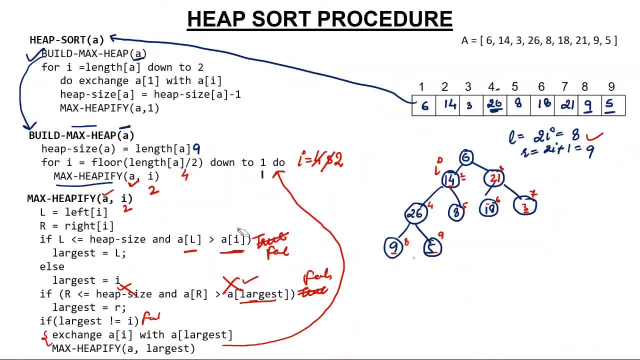 with. I value two, So I will become two. Let me rub all this rubbish. Okay, Let me rub all this rubbish. What will happen? So? L will have left I, So what is left I? This Right will become right I, So this will become R. Is L less than heap size? Yes, L is four and heap size is nine: Yes, 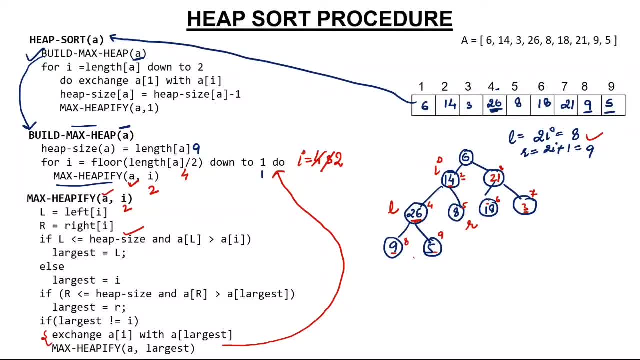 true Is AL. what is AL 26. Greater than AI 14. Yes, This is also true. So the condition become true. I'll move inside and I'll say: largest is L. What is L 26. So 26, that is fourth index. 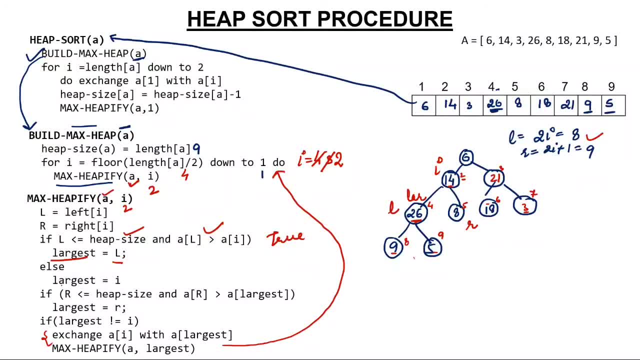 So fourth index is the largest index. No, Again, I'll not move to L's part. Again, I'll say: is R less than heap size? Yes, R is five, which is less than heap size. What I'll do, I'll compare AR with. 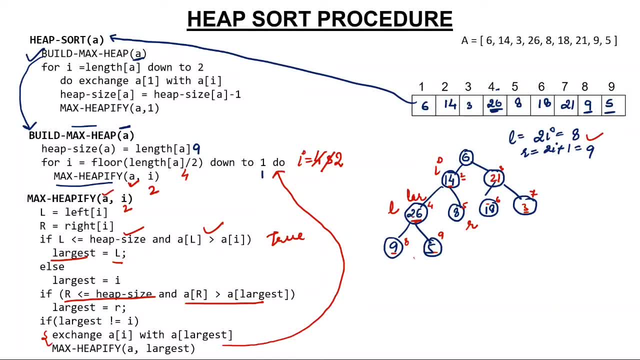 A largest? What is AR? Eight, What is A largest? 26.. Is eight greater than 26?? No, This is true, but this is false. So condition become false. So R will not be a largest. And if this is very true, 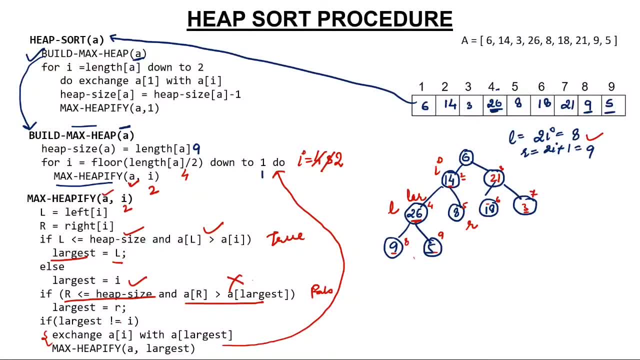 L is the largest. So again, I'll check: is largest not equal to I? Yes, Largest and I are not equal, because largest is at index two, Largest is, as at index four, I is at index two. since they are not equal. So what I'll do? I'll exchange AI and A largest. So when 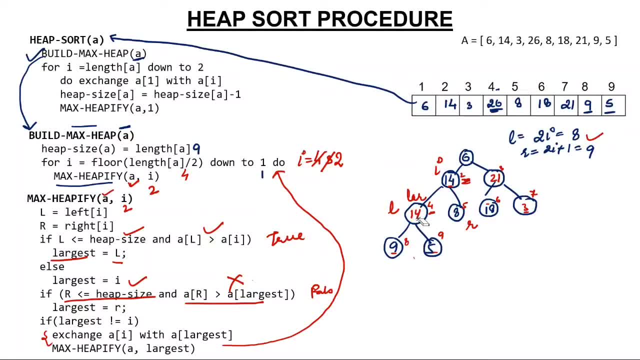 I'll exchange AI and A largest: 14 will come here And this 26 will come here. Fine, 26 will come here. 26 will come here, So 14 will come here. 26 will come here. Now what will happen? So 26 will. 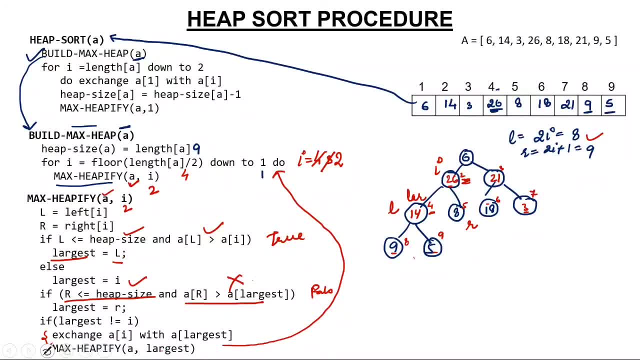 come here. This will come here. Now again I'm calling max heap size with A and largest. What is largest? four. So again I'm calling A with four, four value. This again I'm calling this. what will happen now? What will happen? I will come here because I has now become four. Fine, 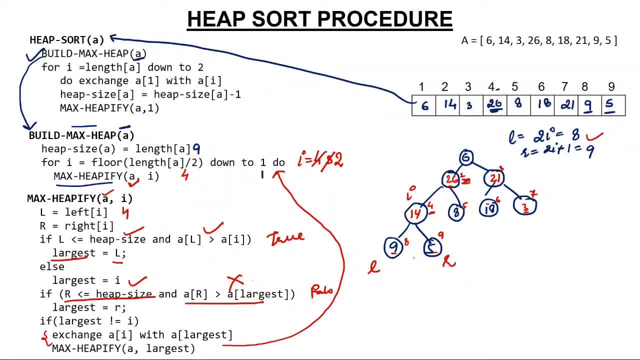 L will be left, I, R will be right. I Again, I'll see this. Is this greater than this? No, Is this greater than this? No, Since both are not greater than this. So this condition will become false. So what will happen? I'll execute L smart, So largest will be I. So this will be the largest. 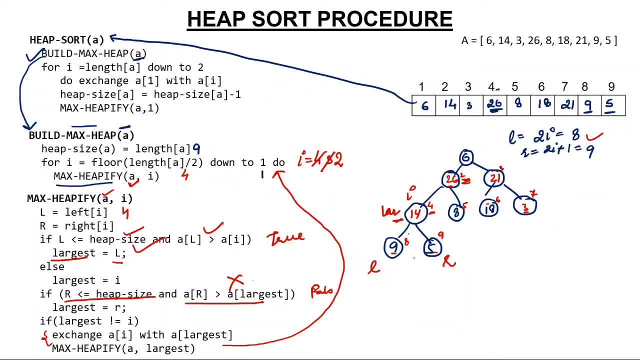 If this is not greater than this, which will be the largest? This Now I'll compare this and this with this line. What I'll do? I'll compare this and this Is this is the largest. Is this is the largest R? No, R is not largest. So this is the largest. Now in if block, I'll check. 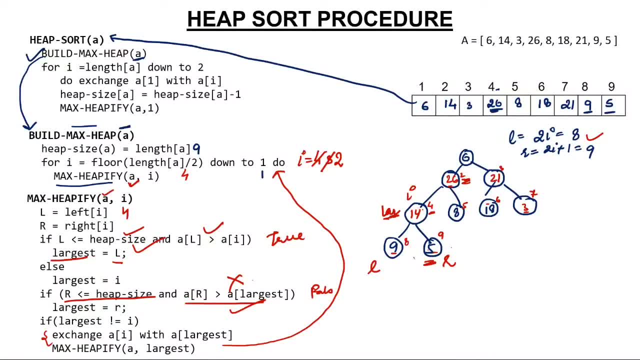 largest and I are not equal. They are equal. I and largest are at same position. So if they are equal, so what? I'll not exchange them. If they are equal, why to exchange? And again, I'll not call them Fine. So till here, my job is done. So till here, till second position. I have done what max. 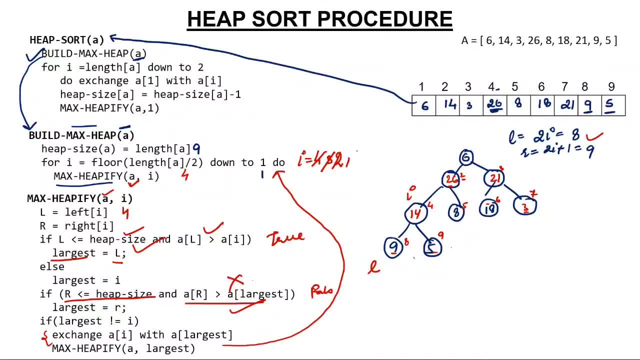 heap size. Is my job over? No, Still, one value of I is remaining. So now final value of I will become one. So again, I'm calling A max heap size with A and I. I is one. So what will happen? 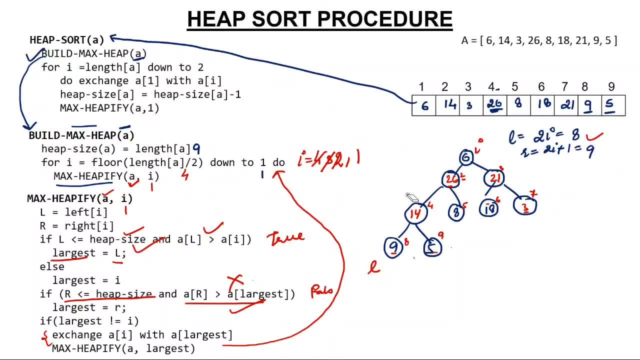 I will become one, So this I will become here. Fine, Okay, So this I will become here. Now what I'll do? L will become left: I. This will become L. This will become right. I. This will become R. 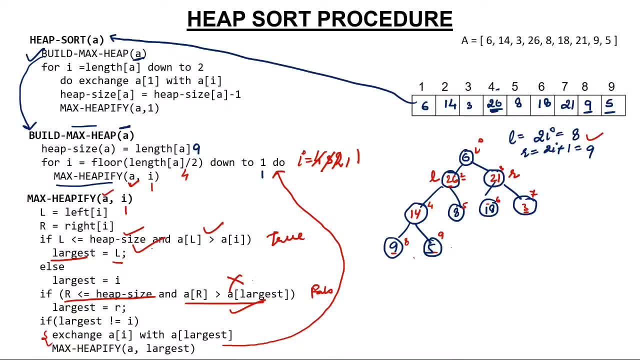 Fine, Okay, Now what I'll do. Is L left hand heap size? Yes, L is at second index. Heap size is nine: Yes, This is true. Is AL this is 26 greater than I? Yes, This is also true. So again, the condition. 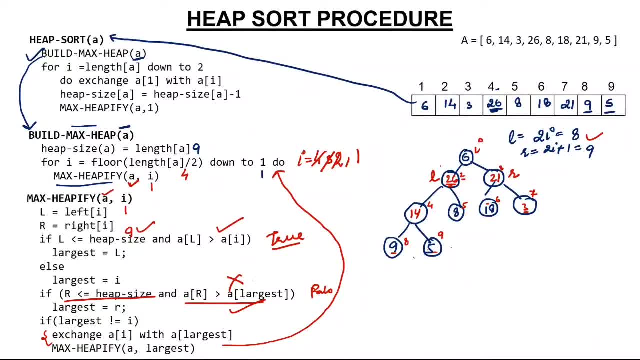 become true. What largest will be? L. So this will be this. L will be the largest. Fine, Okay, This will be the largest. Now what I'll do? I'll compare with R. Is R less than heap size? Yes, R. 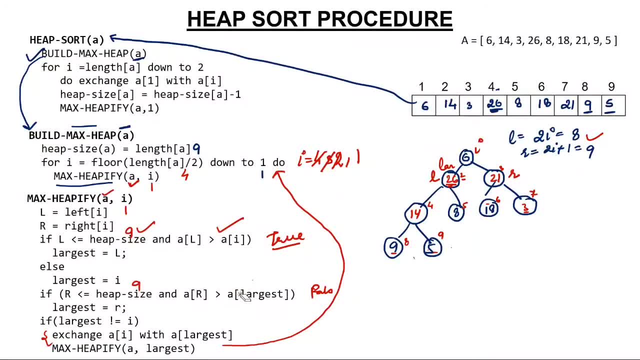 is three. Three is less than heap size. Nine, Very true, Is AR. what is AR 21.. 21 is greater than A largest 26.. Is 21 greater than 26?? No, This is false. So if this is false condition, 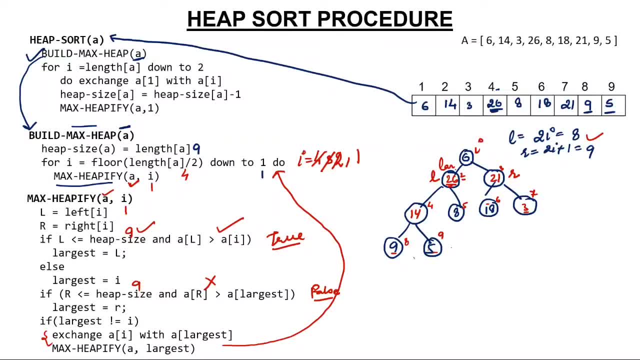 become false. I'll not make largest R, because we know that largest is left only. Fine. So what I do Is I in largest, not equal? Yes, I is at position one and largest is at position two. Since they are not equal, I'll interchange them. So when I'll interchange them? 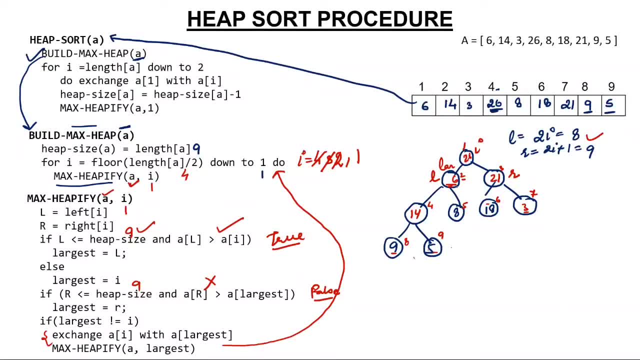 so 26 will come up and six will come down. 26 will come up and six will come down and six will come down. Fine, Okay, Now what will happen Again? see, due to this six, is my property violated. Yes, 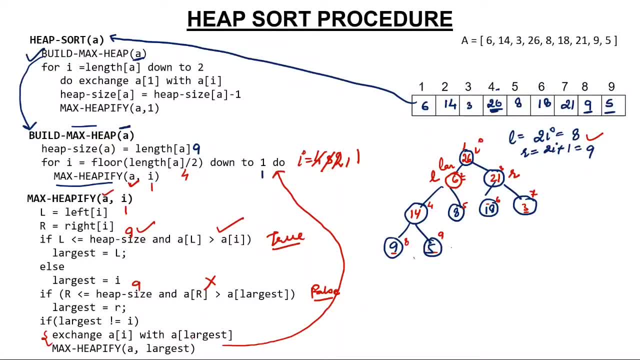 Now, again, I'm calling max heap Y with A largest. What is largest? Two. So again I'm calling this max heap Y with two. See this. So what will happen? This, I become two. So this, I will become two, This, I will become two. What will what I'll do. 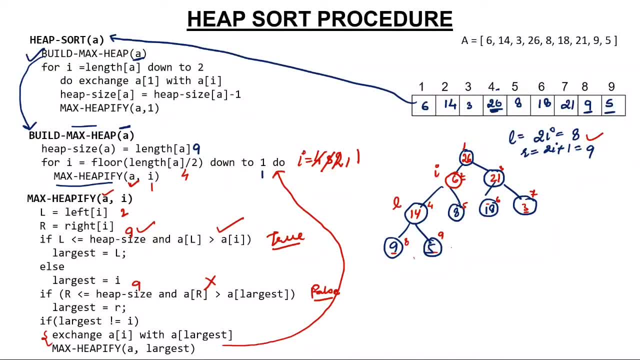 Next, again, L will become left high. This will be L. This will be right. I'll again compare with both the elements. which is largest? This is largest. What I'll do, I'll exchange both of them. So what will happen? 14 will come here, Six will come here. So again, I'll see, So again. 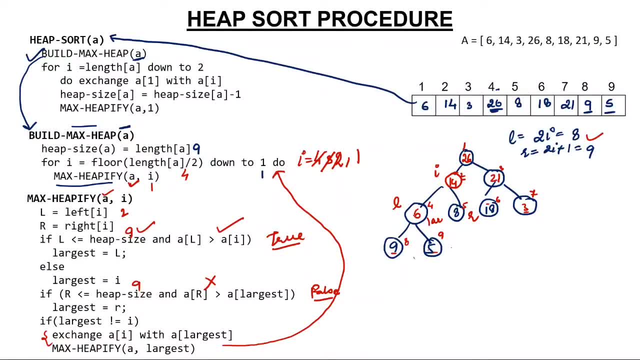 after exchanging, I'll again call A with largest. which one was largest? This was largest, So this will become I, This position will become I, And again I'll check which one is largest. Since this one is largest, what I'll do? I'll again exchange. 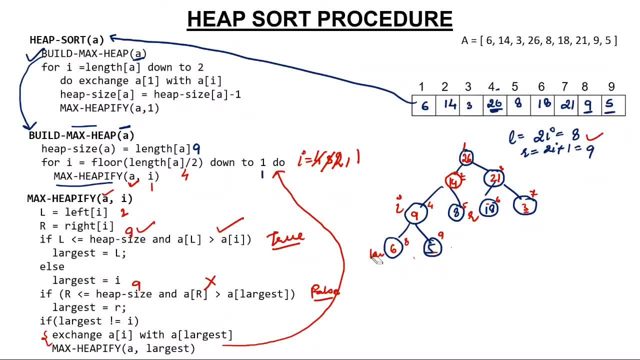 So what will happen? Nine will come here and six will come here. Fine, Okay, So now this again. this will become I. Now there is no element, So condition will become false And finally, I have reached all the condition of I. I have taken all the values of I. Now my job is done. 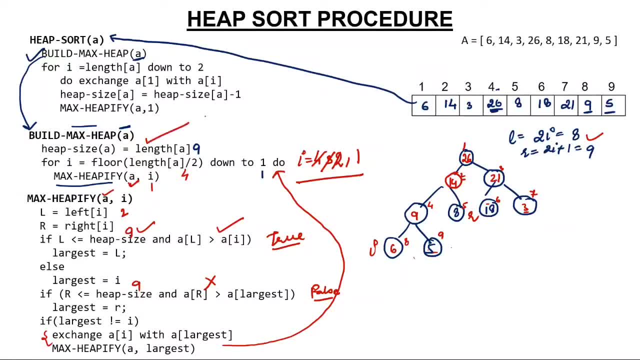 So my build max heap has said: my task is over, My task is over. So now the current tree which you are getting is max heap. So now let me convert this heap to an array. So what will happen? This entire process, this entire element will be changed like this: First, 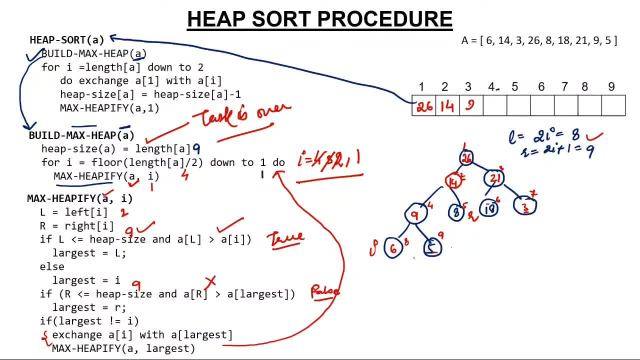 element is now having 26.. Next is 14.. Then 21.. Then we have nine, Then we have eight, Then we have 18.. Then we have three, Then we have six, And then we have five. Finally, we have this. 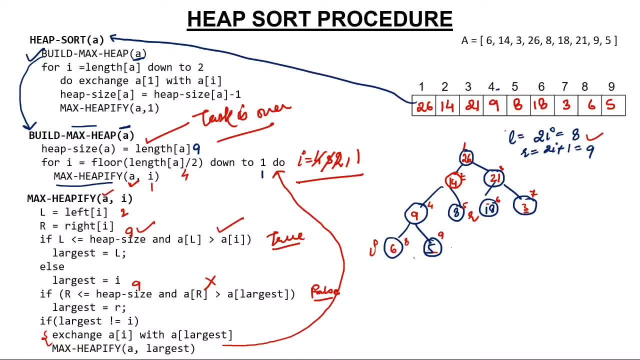 Now, is this a sorted element? No, this is not a sorted element, This is a heap sort. This is not a sorted element, This is a heap sort. So what I'll do next? Now what build max? heap will say: my task is over, So it will again go to the heap sort. It will, since heap sort has. 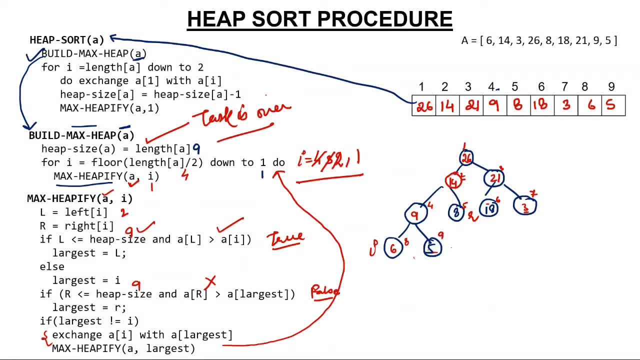 called build max heap to make a max heap. Since max heap has done all its tasks, it will go back to the heap sort and say: sir, you give me an array, raw array, And you ask me for what? Creating a max heap, Your job is done. You asked me to do a max heap, I did it. Now your job is to sort the. 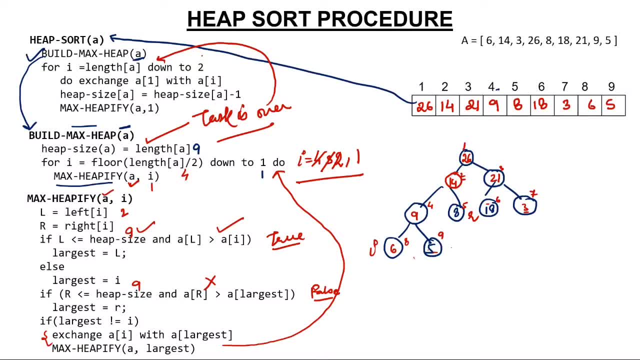 element. So heap sort will say, yes, it's very good. Thank you so much for giving me a max heap. from what Length of A? What is length of array 9?? So what we'll do, it will do. it will start from. 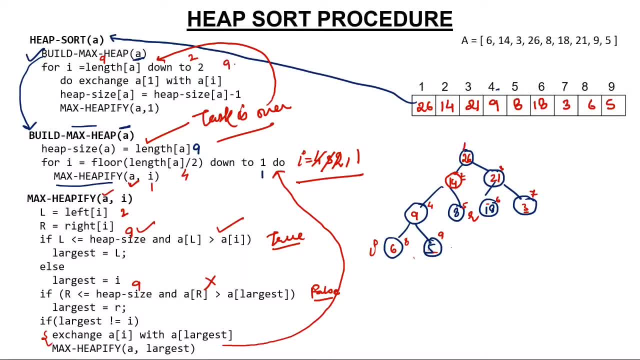 9 till 2.. So what will be the value? 9,, 8,, 7,, 6,, 5,, 9,, 6, 7, 9,, 8,, 7,, 6,, 5,, 4, 2, 5,, 4,, 3,, 2.. 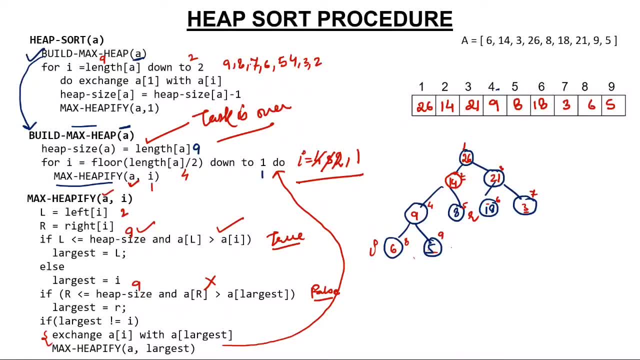 So this will be the accepted value of I. So first I will start from 9.. So it will start from 9.. What it will do? It will exchange A1 with A9.. So when you will exchange A1 with A9, what is actually the procedure? Let me tell. 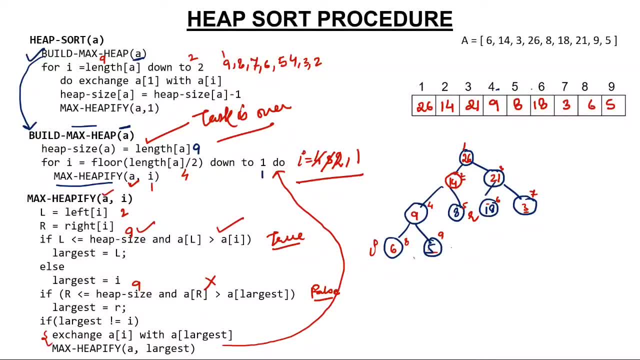 you, Then I'll explain you the algorithm. So how to heap sort is that you exchange first element with last element When you exchange first element with last element, So 5 will come here, 26 will come here and reduce the size and reduce the size. So by doing this you can clearly see the largest. 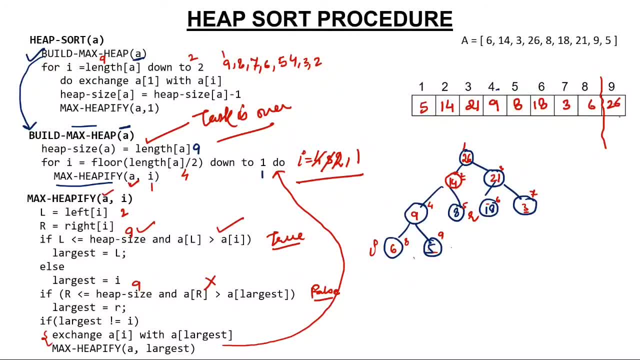 element, The largest element of this array, is at its position. Hope you are getting. It's just opposite to selection sort, So you will do the same thing in the tree. So what you will do: You will replace 26 with the last element, 5.. So what will happen? 5 will come. 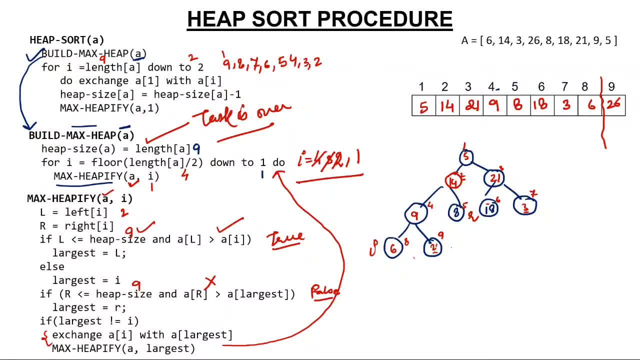 over here and 26 will come here, and then you will reduce the size of heap. So, on reducing the size of heap, what will happen on exchanging? What you will see? by exchanging this heap max, heapify property is violated. You can see that 5 is not the highest element among its both the children. 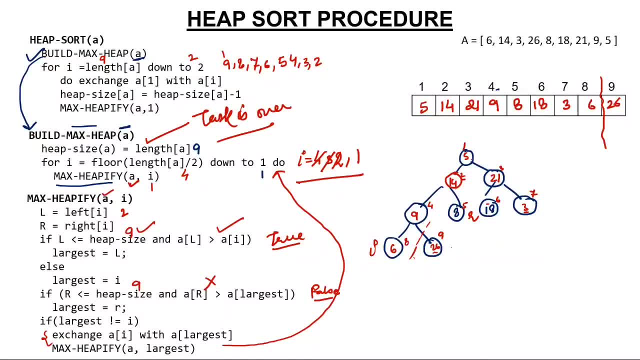 No, it's not greater than from its both the children. What will happen? Again, I have to max heapify From max heapify from where This first position. So what will happen? You will again call max heap from first position. So this will become I, This will become left. 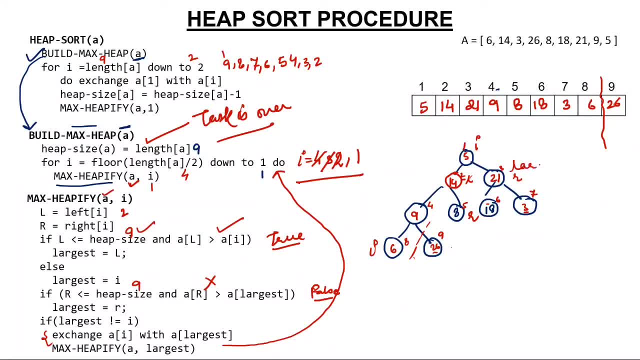 This will become right. Which one is the largest? This one is largest. You will exchange What will happen. 21 will come here. 5 will come here Again. this will become I. Again, you will compare with three elements. Which one is largest? This one is largest because this will become L. This will 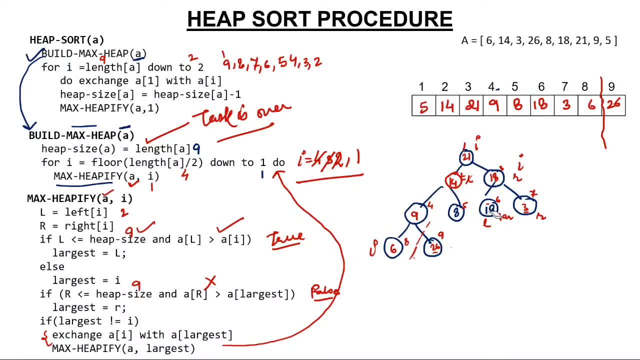 become R, You will again exchange. What will happen? 18 will come here and the element which you have exchanged, which was, I think, 3, whatever it was, It was 3, I think. No, it was not 3.. It was. 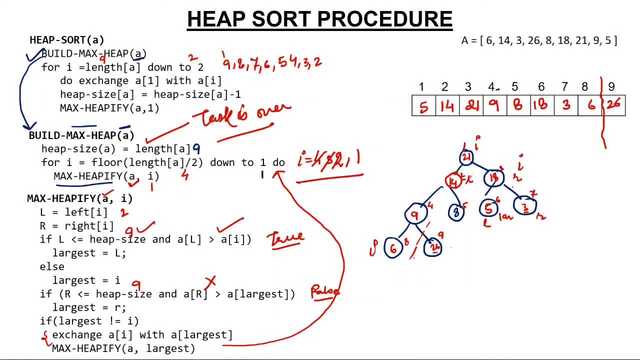 5.. Yeah, 5 will come here, Fine, 5 will come here, Fine. Okay. So now again what we did on max heapify, on calling max heapify: my tree is now max heapify, What you will do, So you will again. 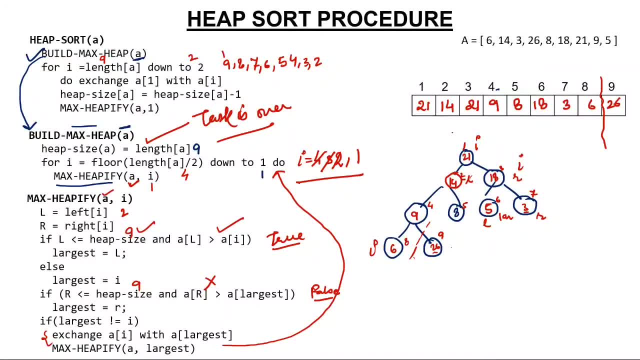 make the changes in array. So first position is now having 21.. Second position is 14.. Third is now 18.. Fourth is 9., Then 8., Then 5.. Sixth position is at 5., 7,, 3. Then 6.. Fine, Okay, Now what you. 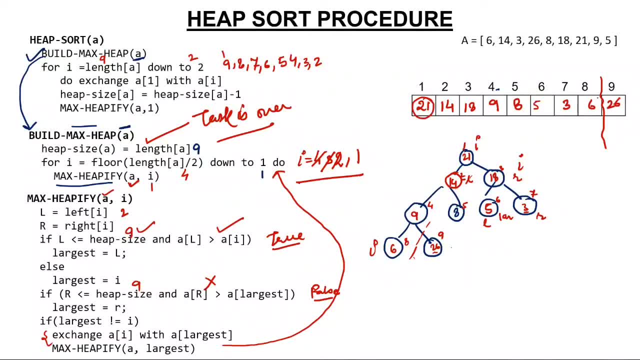 will again apply the same procedure. What you will exchange, You will exchange 21 with the last element. So when you will exchange, what will happen? 6 will come here, 21 will come here and you will see that again. the 21 will come here and you will see that. 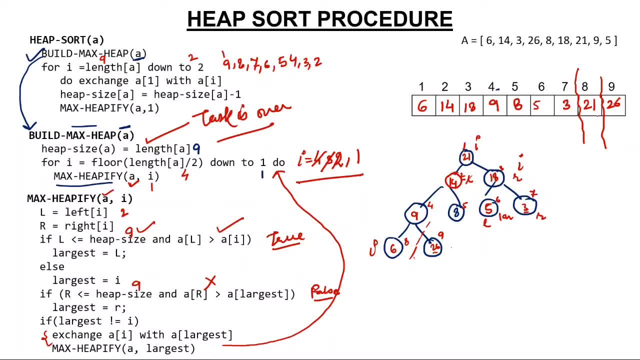 second position is having second largest element. Second last position is having second largest element. You will again make the same changes in the tree also. So what will happen? You will exchange 21 with 6.. What will happen? 6 will come here, Fine, 6 will come here. and what will happen? 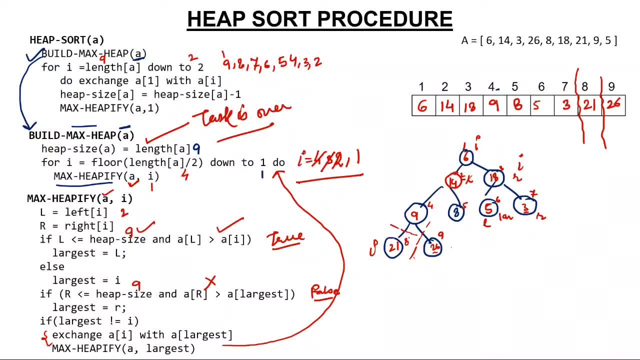 This 21 will come here and you will reduce the size by 1.. On reducing the size, what will happen? You will get 6.. Max CP 5 property is violated. What you will do Again? you will call max CP 5.. 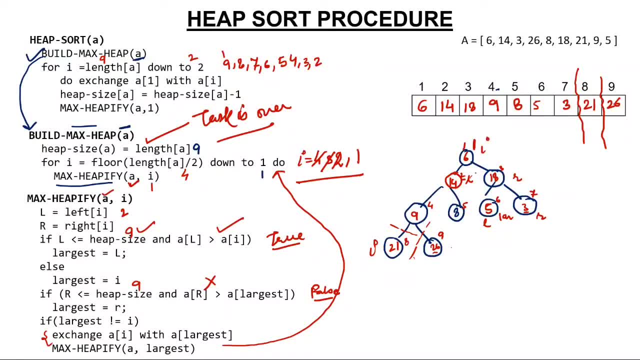 From where, From first value, that I will become 1.. So again you will compare which one is maximum. This one is maximum. You will replace 18 with 6.. Fine, Again you will say this is the left child. 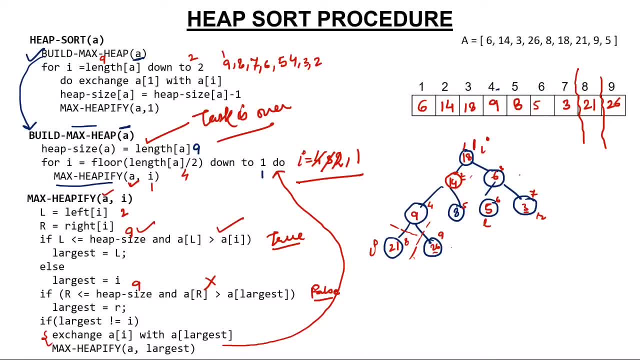 This one is the right child. Which one is maximum? 6 is maximum. You will not do anything. What will be the changes now? First position will have 18.. Second is 14.. Then third will have 6. Then you. 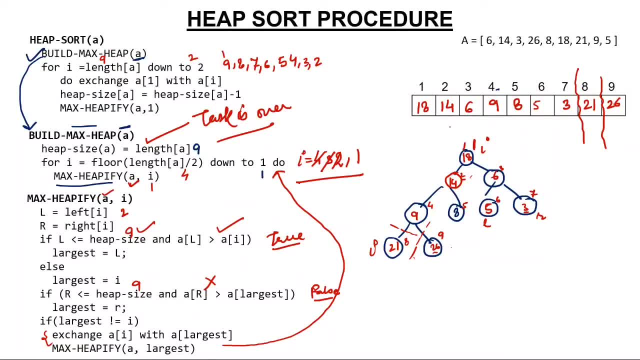 have 9, 8.. Then 5 and 3.. Fine, No issue. again what you will do again, you will replace first with second, the last position, which is last seven. so on replacing, here you will get three, here you will get 18. fine, okay, and you can see the. 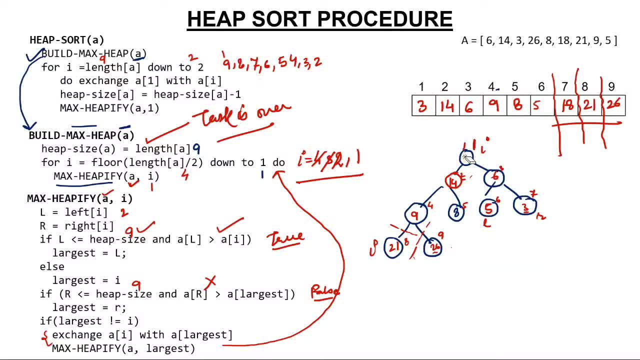 third element: again, you will make the same changes: 18 you will replace with what? 18 you will replace with three. so three will come here, 18 will come here and you will reduce the size. so this is what algorithm is doing. you can see that it's starting from nine. see that it's starting from nine. so the 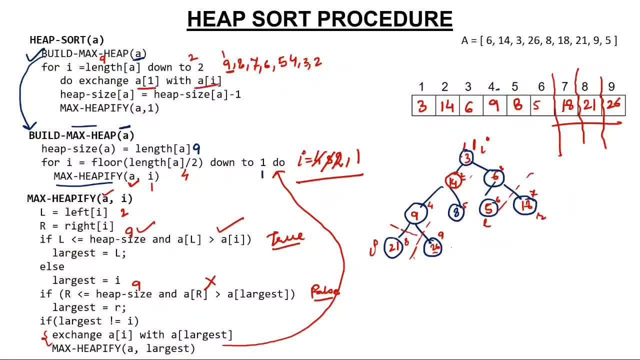 first value of i is nine. so it's exchanging first element with ninth element, fine. after that it is reducing the size, which one which we are already doing. and because we have exchanged it, our max cp5 property is violated. so again we are calling max cp5 with a1. every time you will call with a1. 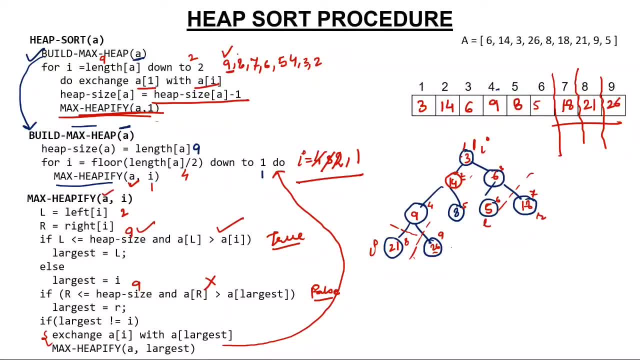 so first you will replace first element with ninth element, then second last with a first element with eighth element, first element with seventh element, then six, and again you will call max cp5 for value one, so on doing this step, finally, what will happen? your array will get sorted. so let me, let me you know, run all these. 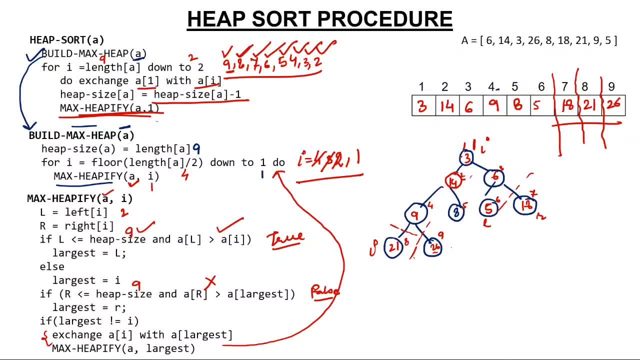 things. now, what will happen and what i'll do? uh three, fourteen, six, so on. uh three, since three violates, since three is violating the property. which one is maximum? this one is maximum. so what will happen? uh, 14 will come up, three will come down. i'll again see which one is maximum. this. 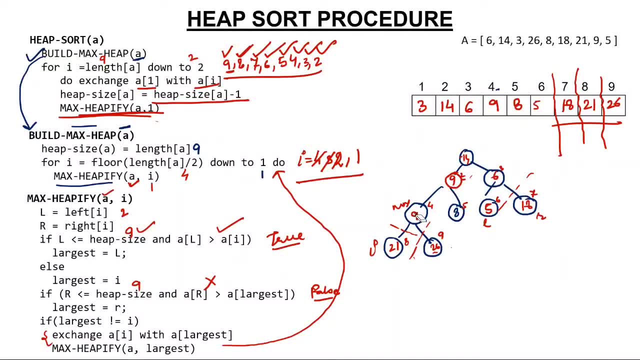 one is maximum. what will happen? nine will come up and three will come down. so since there is no element after that, what will happen? i'll make the changes in array 14. second is nine, third is six, then, uh, fourth is third, three, fifth is eight and sixth is: 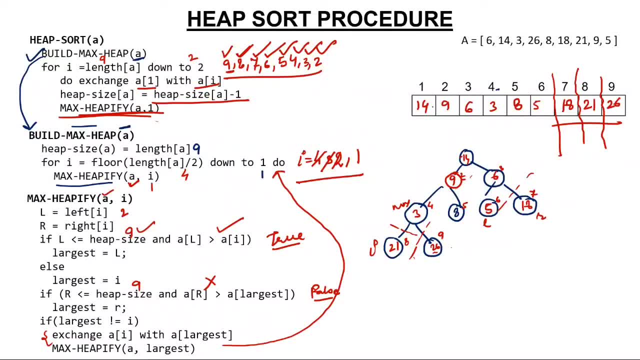 five. fine, okay, now you have again made the changes. again what you will do: exchange first element with last element. so when you will exchange, five will come here, 14 will come here. you will reduce the size. you can see that clearly. your element are started sorting from- uh, backside. fine, so what? 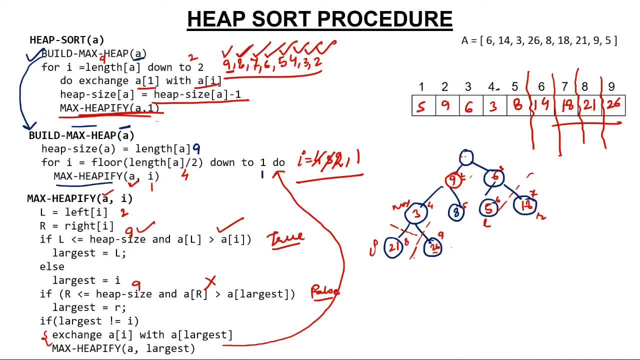 you will do when you put in three. also, you will replace 14 with five. so five will come here, 14 will come at six. this position, fine, and you will reduce the size. fine on reducing what happened, on exchanging what happened, that the five is violating the property of maxi. what you will do. 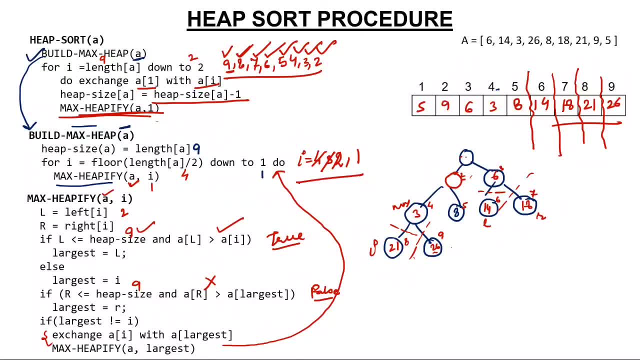 again, you will find the maximum. this one is maximum. you will replace nine with five. again, you will see which one is maximum. this one is maximum. it is maximum. it will come up, five will come down. fine, so what happened? what changes took place? nine will come here, eight is at second, six is at third. 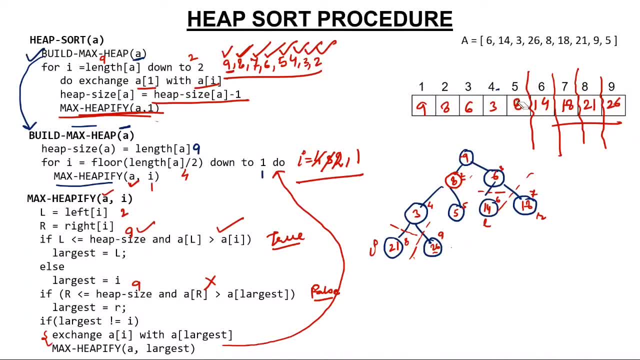 the fourth position has three, and fifth position has now five. fine, okay, now what you will do. again, you will replace first with last element. so when you will replace first with last, and when five will come here, nine will come here, you will reduce the size. so again, you do the same thing in three. 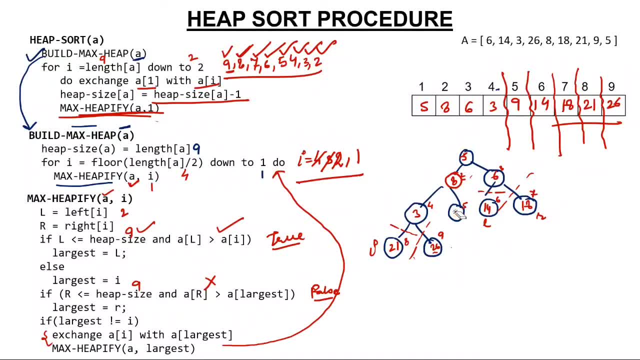 also what you will you do. you will replace five with nine. you will reduce the size. on making the changes, is your properties violating? yes, you will again see the maximum, which one is maximum. eight is maximum, so eight will come here. five will come here again, you will see, since there is only the 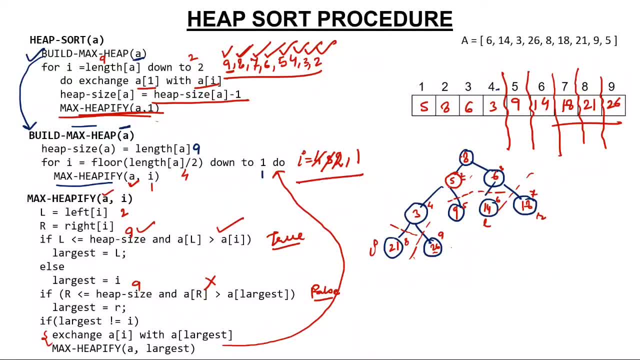 only one element. you will compare. since five is at its correct base, you will not do anything. what changes took place? eight has come here, then five, then you have six, and then you have three, six and then three. fine, okay, what you will do again? you will replace first with fourth element, because 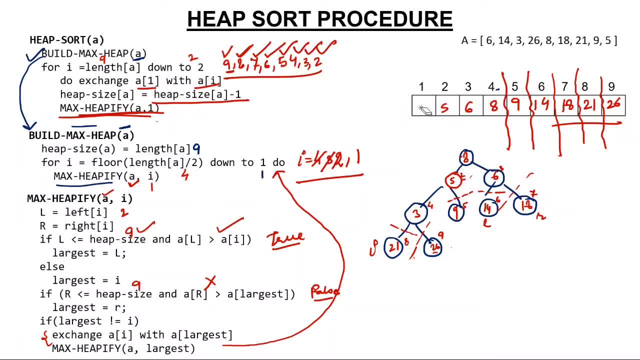 it is at I fourth. so what will happen? eight will come here, three will come here and you will reduce the size again. what you will do? you will replace eight with three. that is entry. also, three will come here. it will come here. you will reduce the size on making three at upside. what? 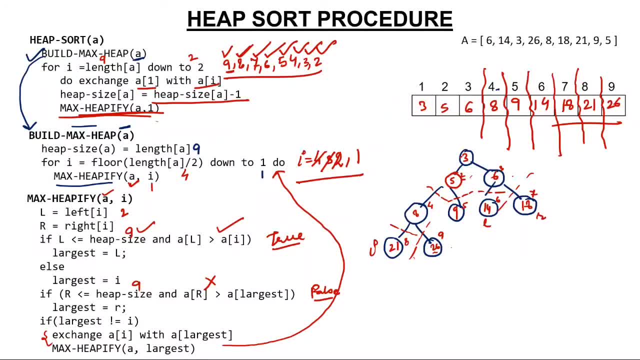 will happen. see, is trees violating property. yes, which one is maximum? 6 is maximum. 6 will come here. 3 will come here. there is no element. you will not do anything. what changes took place? 6 came here. 5 is at its place, same place. 3 came here again. what you will do, you will replace, you will you. 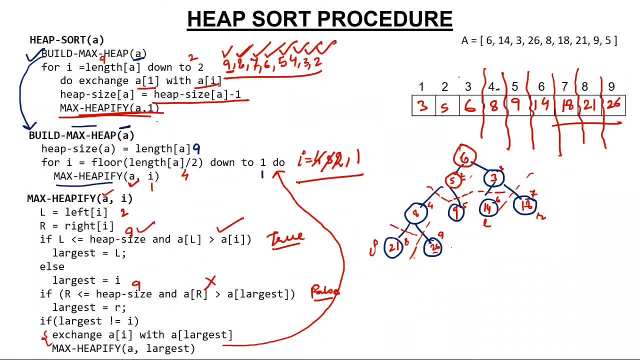 will exchange first with last. so 6 will come here, 3 will come here. you will reduce the size, so you will reduce the size. so what again you will do? 3 will come here, 6 will come here and you will reduce the size. fine, now you have left with only 2 element. now you can see that loop. 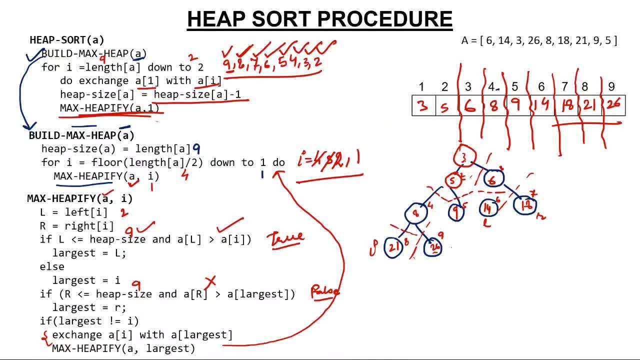 will only move to second position only. is this properties violating? yes, so 5 will come here, 3 will come here, fine, okay. and 5 and 3, and you will reduce the size. so what will happen? you, I am so sorry. 3 and 5, yes, it will exchange and you will reduce the size until second. 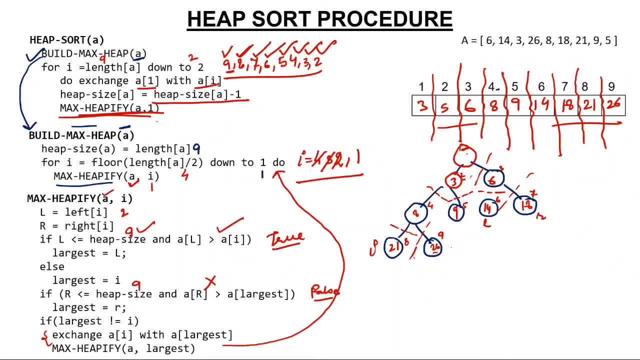 your entire work is done. fine, so your entire work is done. so what will happen? 5 will come here, whatever it is, and your job is done, and you will reduce the size, something, something like this: so sorry, three will come here, five will come here and you will reduce the size. so three has came to its proper place.